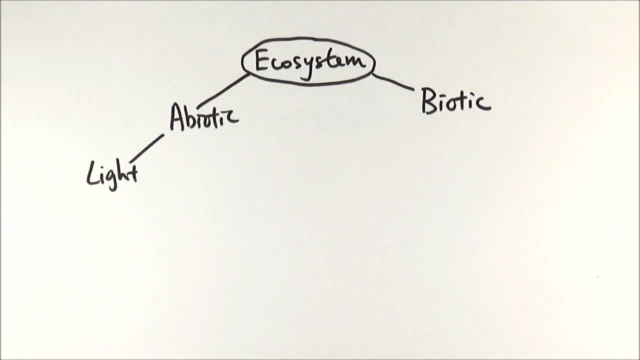 so that is definitely one thing that will affect the amount of plants, shall we say, or the growth of plants in an ecosystem. Photosynthesis also needs other things, for example water. So water availability or water levels in a particular ecosystem can make a major difference in an ecosystem. So we'll be 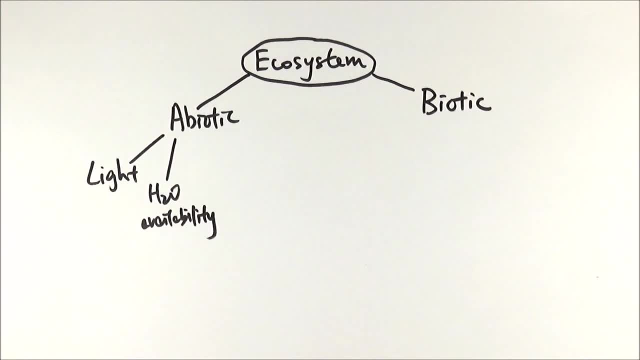 looking at an example of a plant that's not very polluted and has a very massive impact. so an area with lots of water would promote plant growth, whereas an area with less water will have less plant growth. Another thing to consider will be oxygen availability, because obviously all living organisms need. 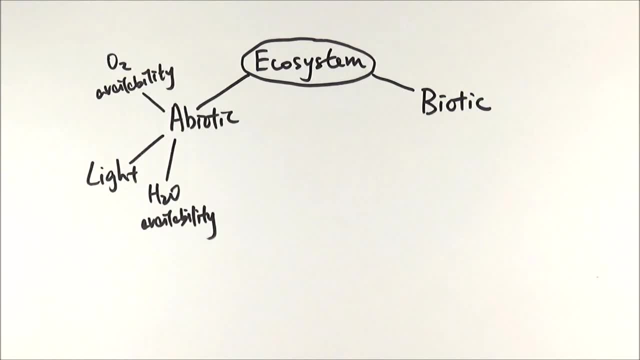 oxygen to do respiration. so therefore oxygen levels are really, really important in an ecosystem. There are two more things, one of which is temperature, and obviously temperature can affect enzymes in our body, which is quite an generation which changes the population size in different areas. So that's another thing to. 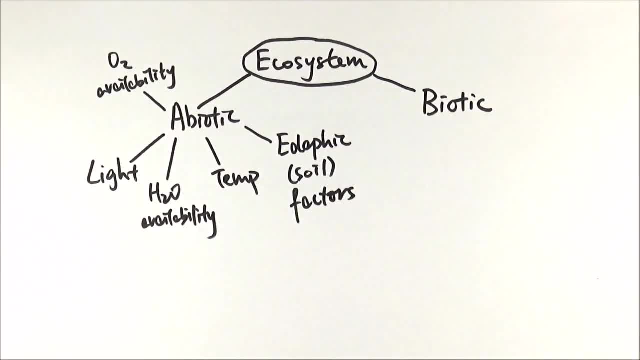 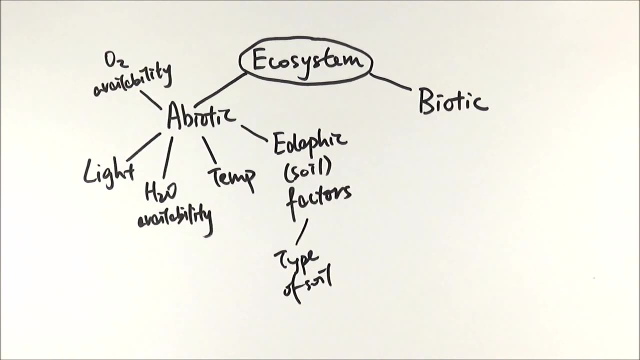 consider. Finally, we have daphic or soil factors, and there are two types. So, thinking about this, we can say the type of soil would have an impact on the types of organisms or types of plants that can grow. So, for example, certain types of soil will be better at retaining water, which is good. 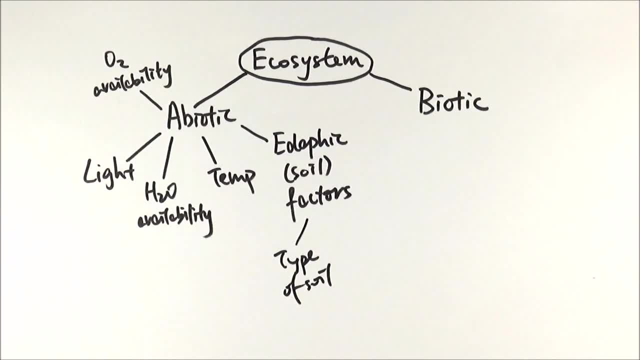 for the plant, and some of them would not be so good at doing that. However, there are obviously soil that are so good at retaining water, meaning they are decreasing the amount of oxygen available as well, which is not great, so you want something that can have a good balance. Another thing we can: 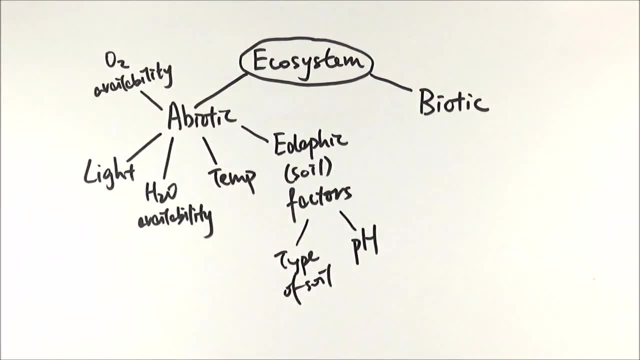 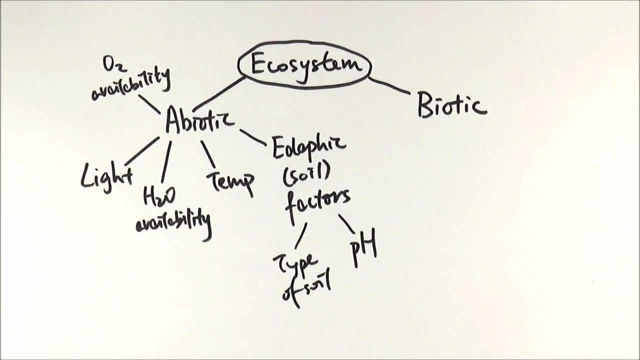 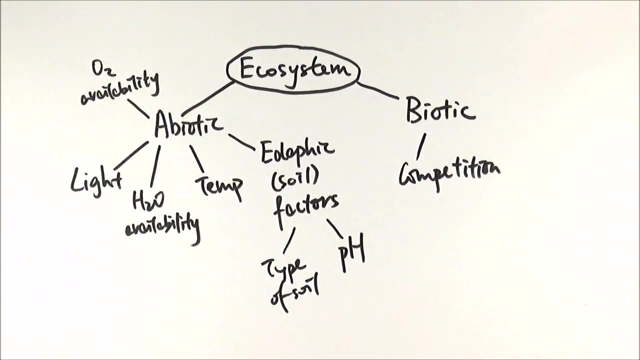 consider will be soil pH, because different plants would prefer different pH levels, so it's important to keep an eye on that one as well. So now we'll have a look at biota factors, and actually there are only three key ones that we always consider. The first one is competition. So in an area where 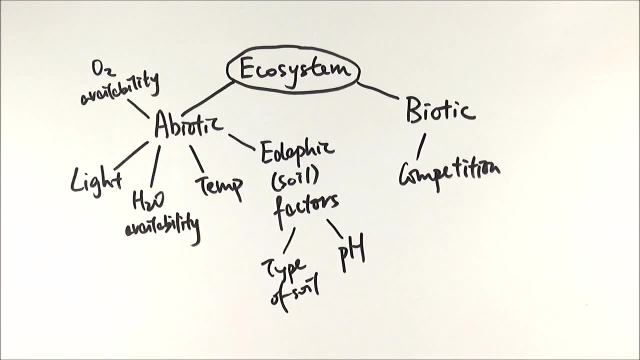 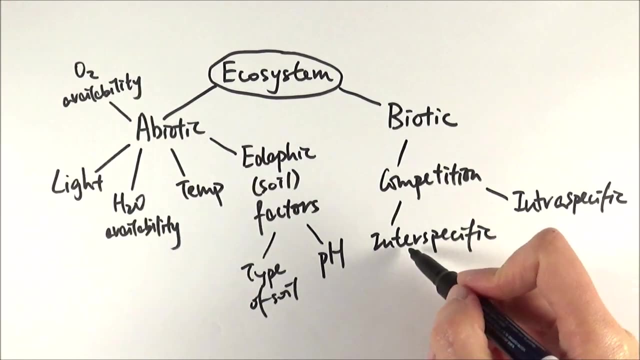 you get different organisms, they would obviously be competing for the same resources. So, for example, the same type of food, the same space or even the same mate. And there are two types of competition which we can discuss more in chapter 24.. That is interspecific and intraspecific. Notice the difference between the. 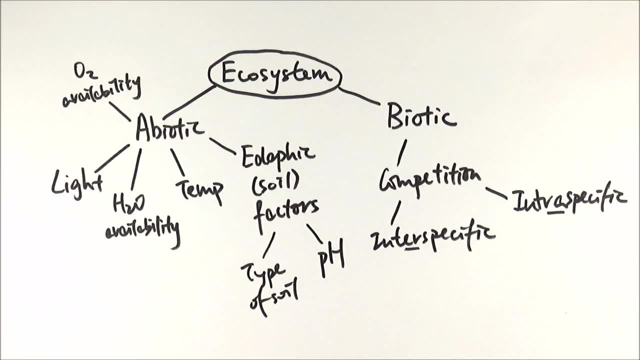 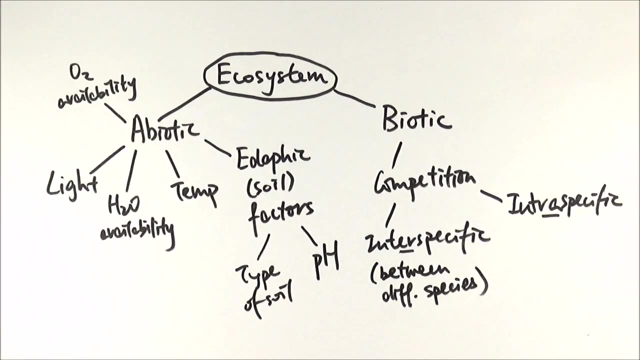 two, So interspecific. think about international. So international it means between different nations, different countries. So therefore interspecific refers to competition between different species. Intraspecific- I think about intranet- refers to a closed network where only selected people can have.